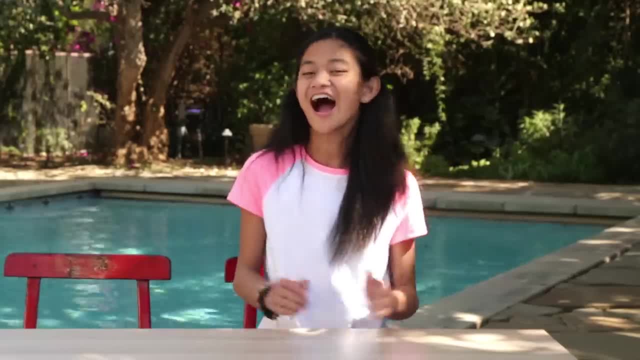 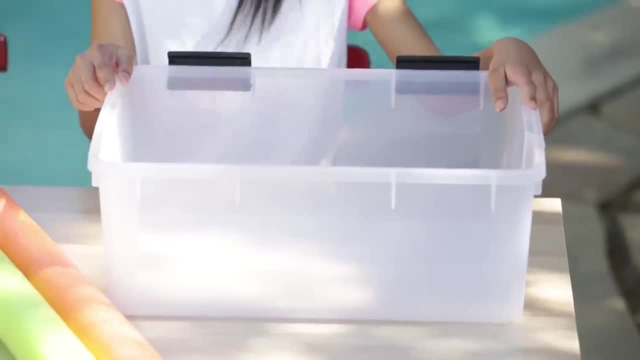 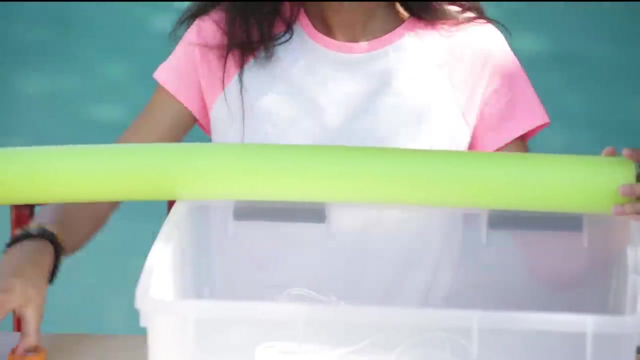 And get something to drink. Well, lucky for you, I was going to make my cooler noodle cooler. For this hack you'll need a plastic storage container that isn't too deep, two pool noodles, waterproof rope and scissors. Cut two pool noodles that are equal to the length. 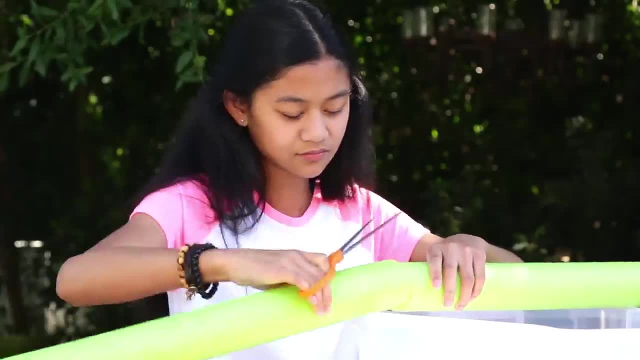 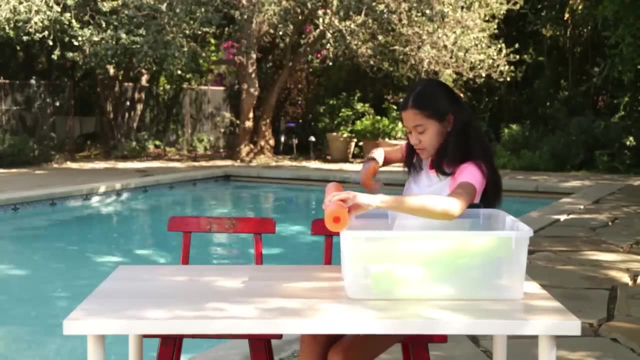 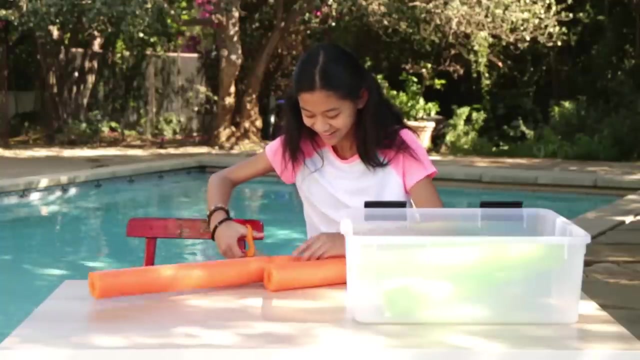 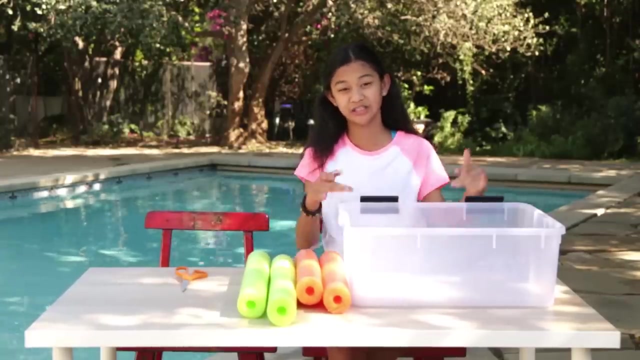 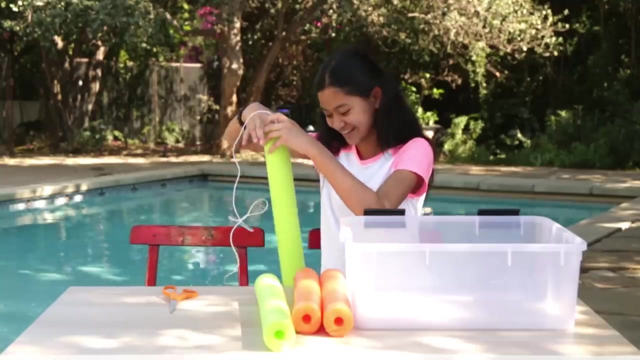 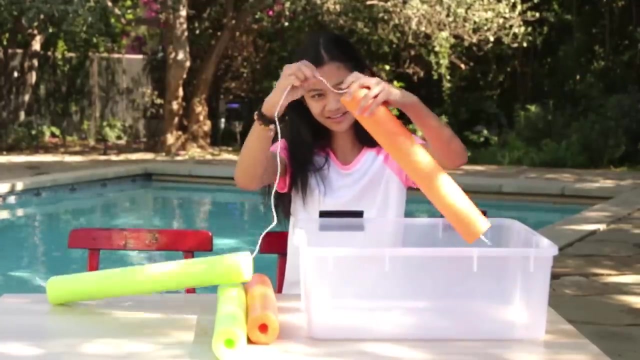 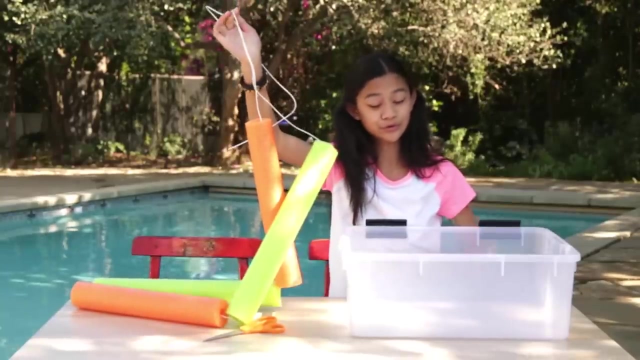 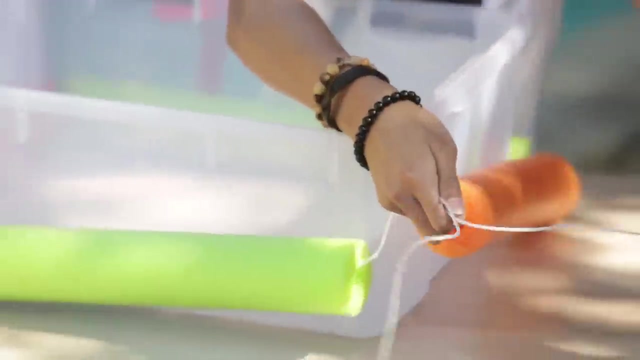 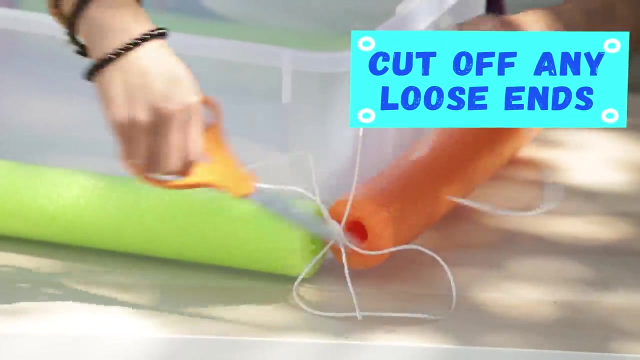 and two that are equal to the width. Now thread your rope through all four pool noodles, alternating between the length and the width. Now wrap your pool noodles around the lip of the container and tie it in place. Now just add ice and your drinks are ready to set sail. 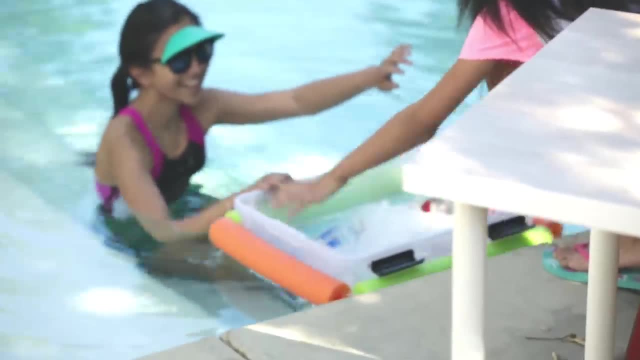 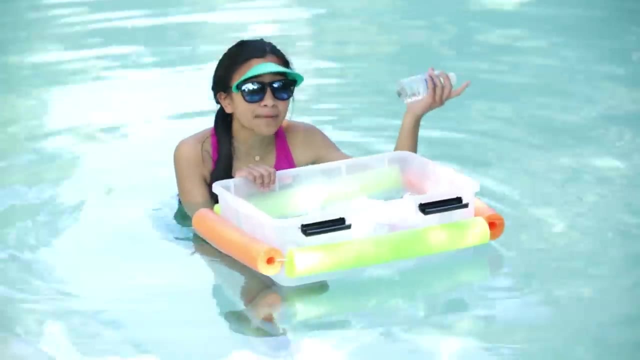 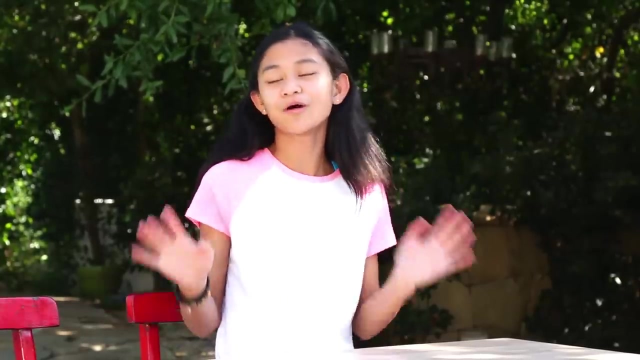 Here you go. Thanks again, You're welcome. But, Jillian, What now? You call this kicking back at the pool hacks? but so far, all we've done is work. Yes, all we've done is work. Well, don't worry, because you'll be relaxing on your back. 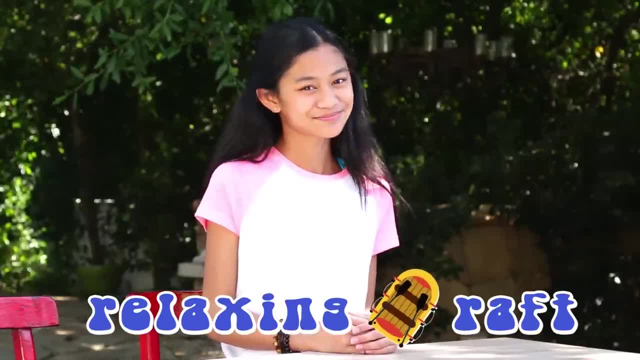 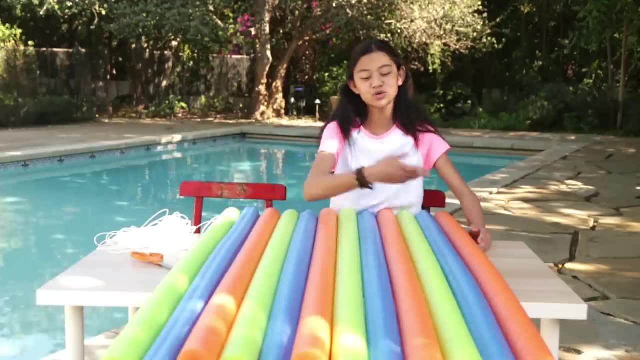 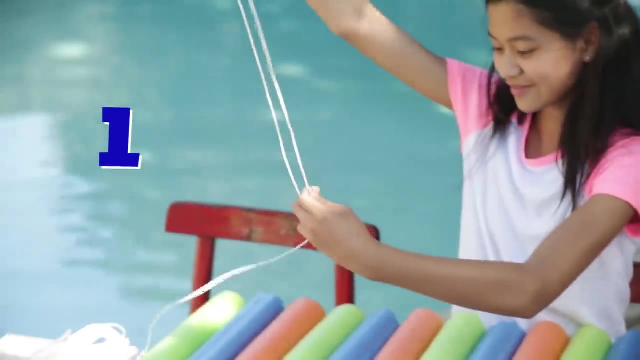 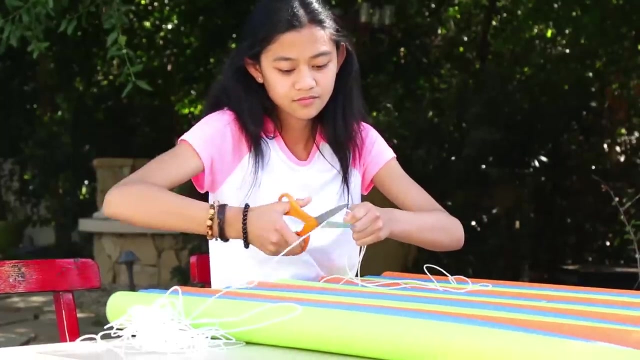 and no time flat with my relaxing raft. For this hack you'll need 12 pool noodles, waterproof rope and scissors. Lay out your 12 pool noodles like this: Now: take your string and measure about three times the width. Fold your rope in half. 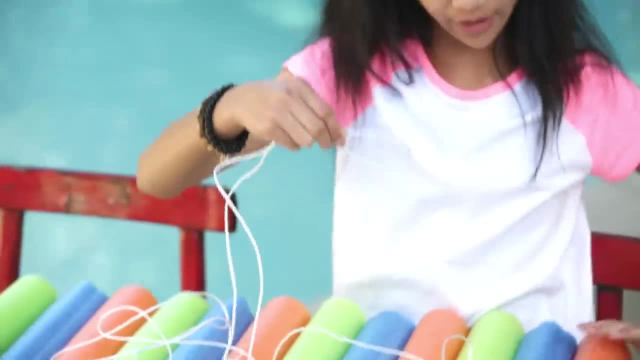 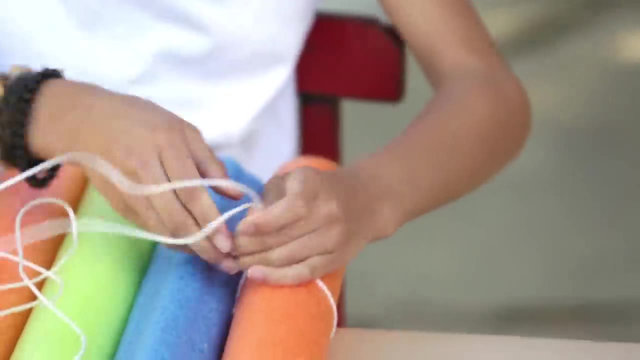 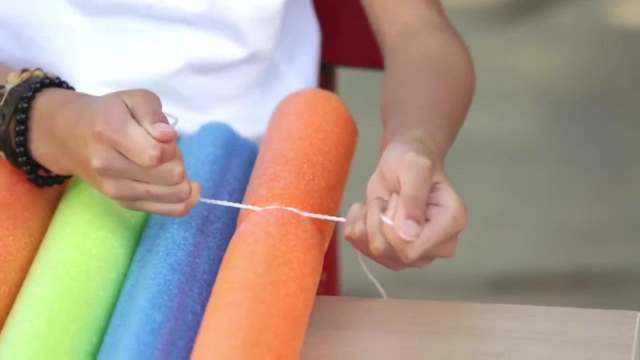 And then, where you folded it, wrap it around the end of your pool noodle And make sure to push it about six inches like this, And then tie one knot, Pull it kind of tight And then repeat this step for the rest of your pool noodles.